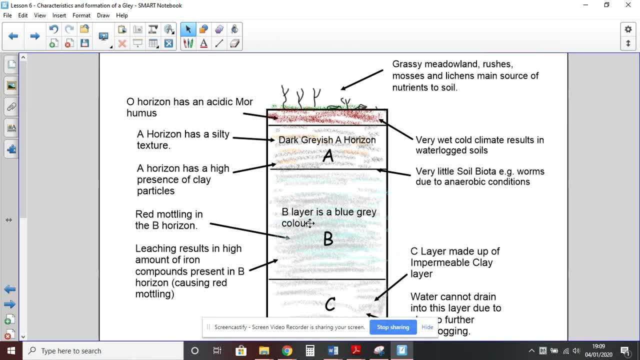 the world. It's obviously associated with Scottish bogs and upland mountainous areas that are very wet. It's pretty infertile. farmers don't typically use it for anything other than rough grazing at best. Okay, so what I need you to be able to do is probably be able to draw this diagram to answer. 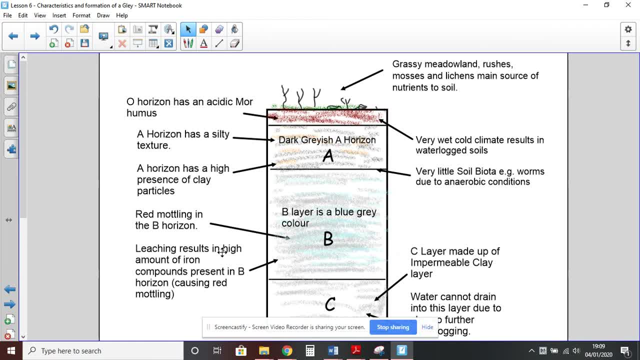 the first of the possible exam questions, which is drawing and annotating, and then, once you've learned that diagram, look to be able to explain each of these points. Okay, and that's what I'm going to do with you now, step by step, and after each step, I would suggest you pause it, note down. 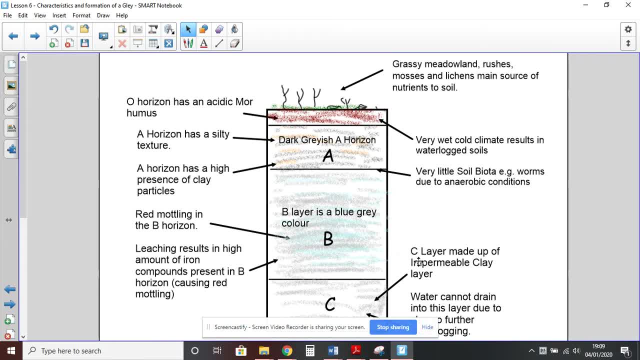 the explanation along with the point of description, and look to build sort of five or six of these into a good answer. Okay, so the first thing you're going to want to say is that these soils form on poorly weathered parent material and then you can say which results in the soil being very poor in mineral content. So that would 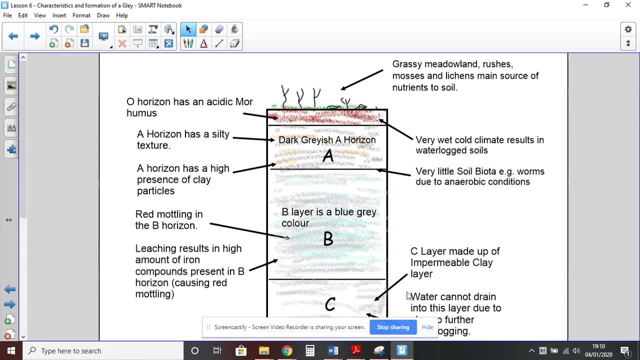 be poorly weathered material as a description and then explaining that this then results in the soil being very poor. A poor amount of minerals would be the explanation of how it contributes to the soil Sticking with the parent layer. we could then go a little bit further and say the soil also forms. 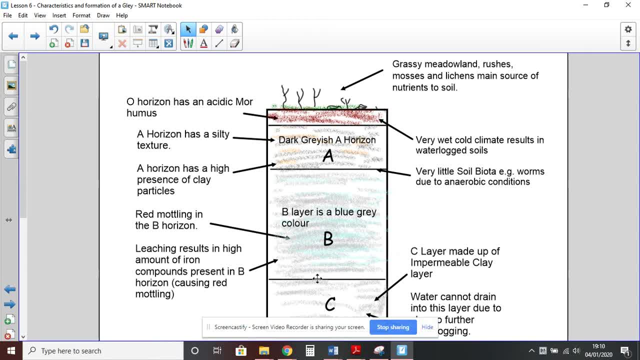 often on clay- which will stop the downward percolation of water, because water would be percolating downwards- well, would be reaching downwards- and when it gets to the rock layer it would either percolate into the rock or, if it was impermeable and it wouldn't. But because clay is impermeable, it cannot percolate to water. 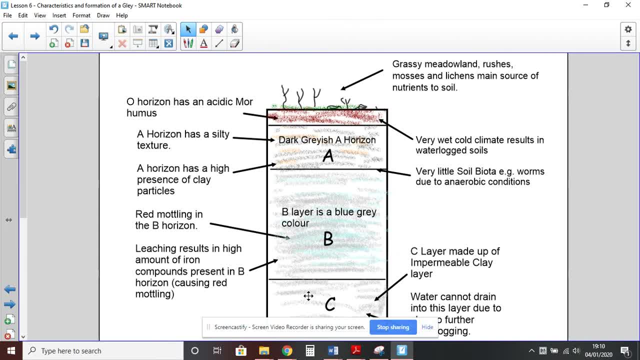 percolate into that rock. so that's the first thing you'd want to say: that it forms on clay, which stops percolation of water downward. now to explain that, you would then say: which results in the soil becoming waterlogged because the the water can't percolate into this sea layer. okay, so there's your. 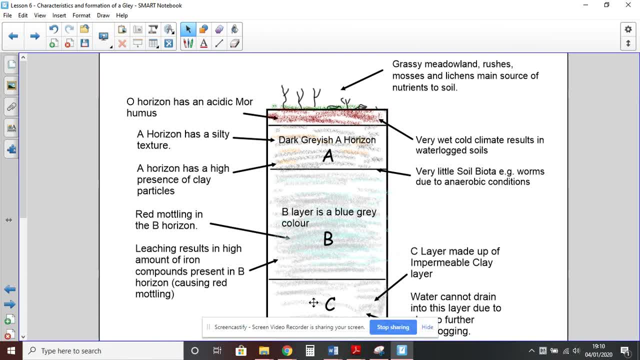 second point. now, if we move on to some other points you can talk about, you can say that the soil is also going to be very waterlogged because it's found in very wet climates, like the mountainous areas or river flood plains, or at the bottom of the slopes, meaning that there's a huge amount of 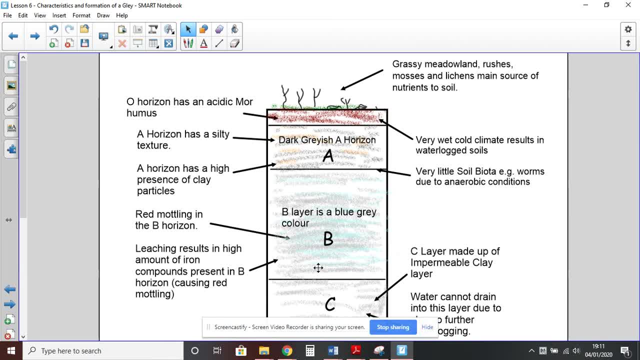 water building up in the soil all the time and because it's also a cold climate, there's going to be very little evaporation of water out of the soil. another point you can make is that the soil is poorly mixed and you don't want to explain that, and you would say that's because of a lack. 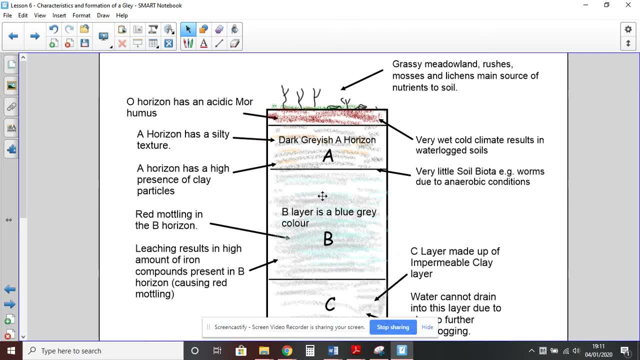 of soil biota, for example. once- okay, developing this idea into another point, you could say: the soil lacks biota. and now you want to explain why it lacks biota and you'd say because it's found in very cool climate, cold climates, so therefore it's difficult for organisms to survive, and also because 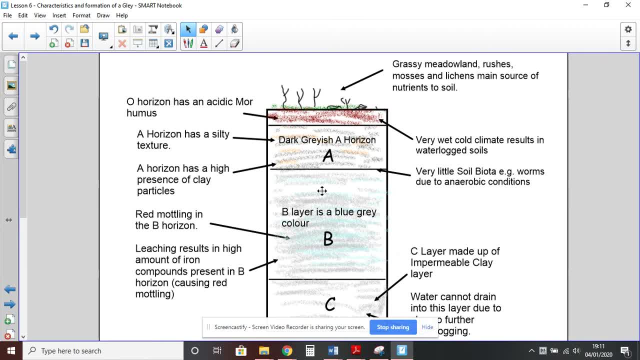 it's waterlogged. this creates anaerobic conditions, which means that there's very little oxygen in the soil and therefore soil organisms, or biota, which is a better word to use, cannot survive. okay, the top layer, the o horizon, is very dark and it's an acidic moor humus. that's emery humus and it's very 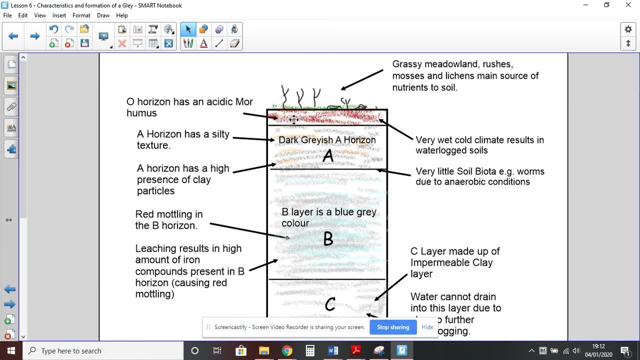 dark and acidic moor. to explain that, you'd say that's because there's a very thin natural layer of vegetation, like mosses and lichens, which is why it becomes very dark and acidic. you can also make a point here of saying that because there is a very poor vegetation layer on the surface. it 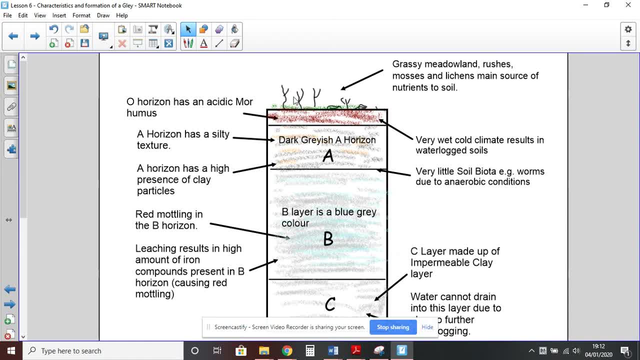 results in the soil being very nutrient poor because there's very little nutrients being leached downwards, because the organic layer is very poor in nutrients. okay, a few other points. the soil tends to be very thin, it's not, it's not very deep, and you would then say this is because it develops in very cold climates where there's limited natural. 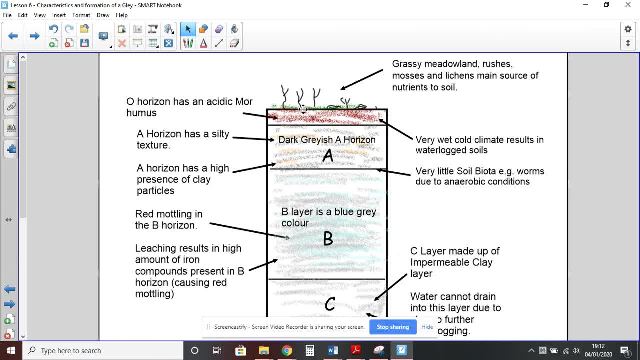 vegetation growing, which would have otherwise fed the soil, but because it's very cold, very little grows on the surface and therefore the soil takes a long time to develop. finally, you can tell me that heavy rainfall reaches the upper layers, the a horizon, giving it a sort of 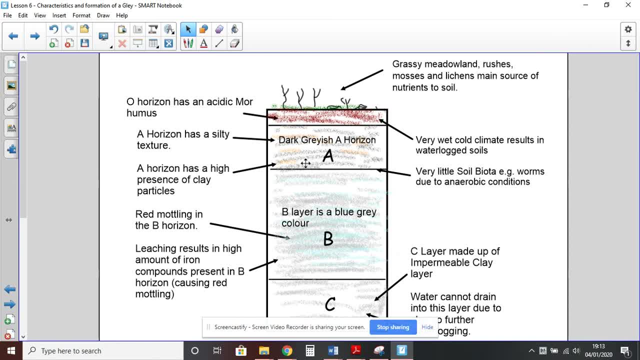 dark grayish color and the iron compounds present in the soil get mainly leached down to the b layer and then they oxidize, which is the same as rusting, which is why the b horizon often has a kind of reddish mottled. look, that's this kind of speckly red. look, if you were to dig into it. okay, so we've.